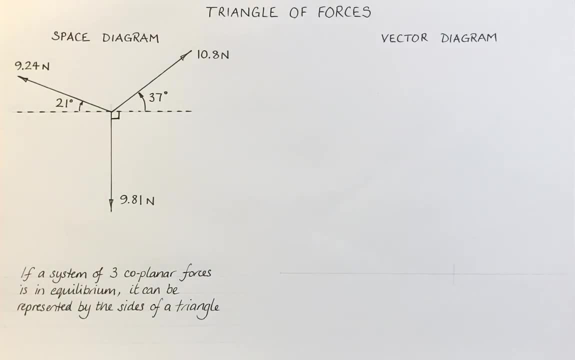 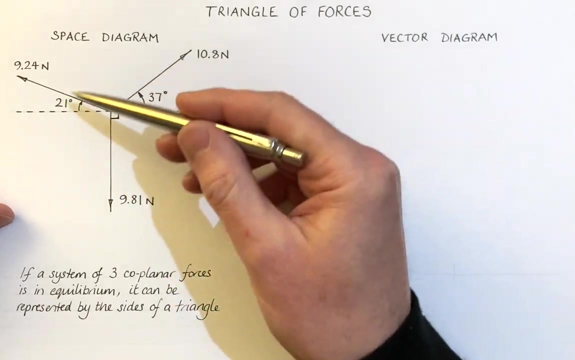 Hi, this is a short video to show you how to draw a triangle of forces vector diagram. A triangle of forces vector diagram is a representation of a system of forces And if a system of forces and their coplanar forces are in equilibrium. 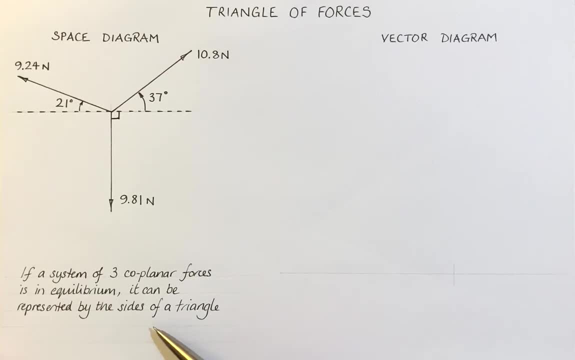 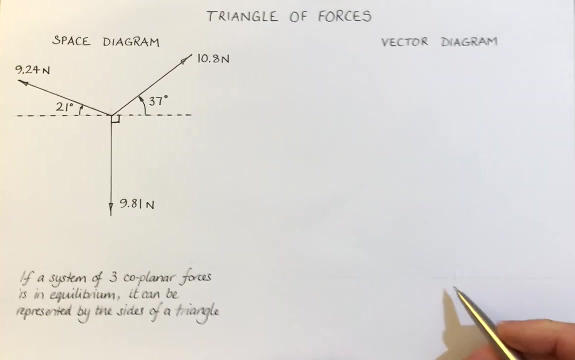 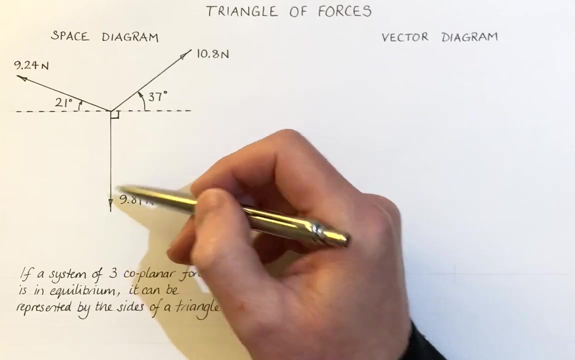 the system can be represented by the sides of a triangle, And that's what we're going to do over here. First we draw a horizontal line with a starting point and then we're going to draw our first vector. Our first vector is going to be this one here: 9.81 newtons acting straight down. 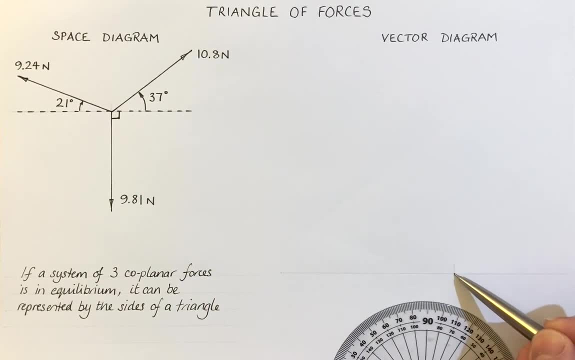 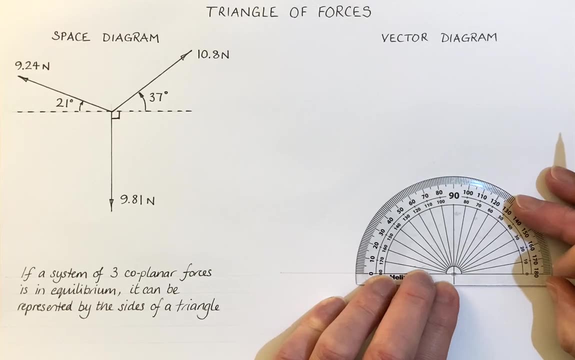 So I take my protractor over to our starting point here and I carefully measure around to 90 degrees. I'm just like that, Lining up the protractor with the crosshairs, the line at the zero there and the line at zero there, to make sure it's placed accurately. 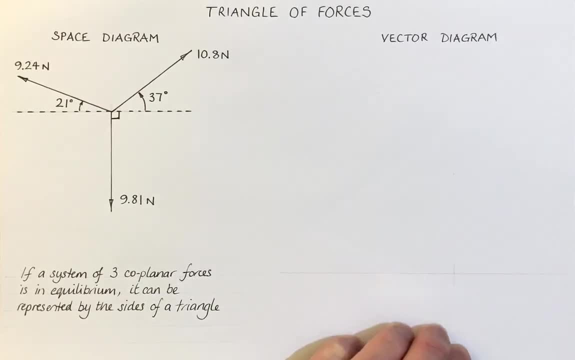 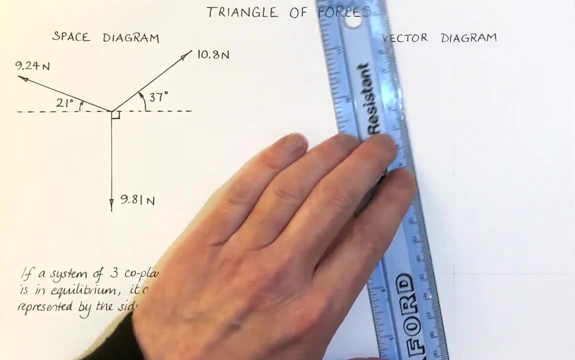 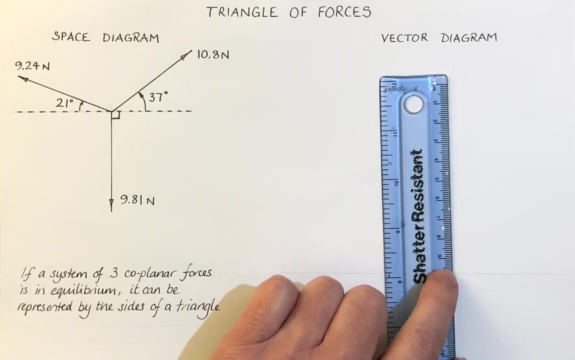 And then I'm going to make a mark at 90 degrees and join that up with a very faint line like so: Now it's 9.81 newtons, so we need to think about scale. So I think one newton per centimetre. 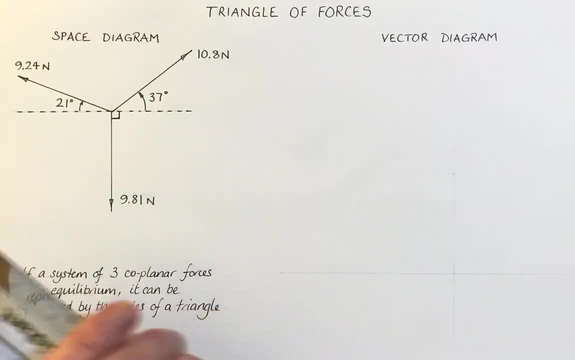 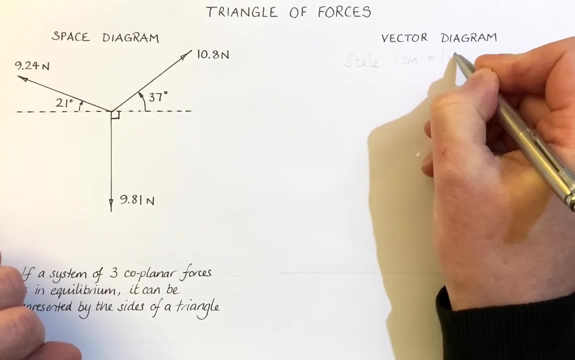 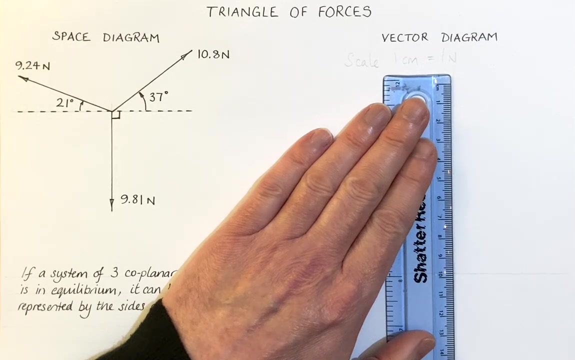 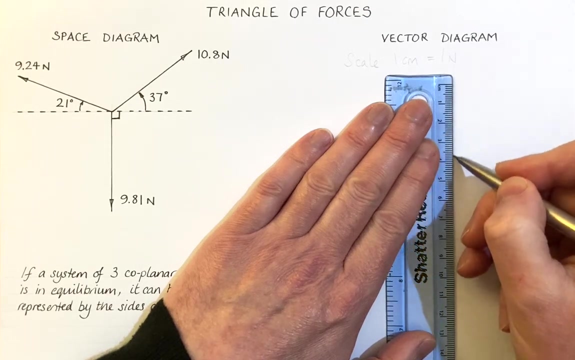 One centimetre should suffice there. Let's write that up Scale: one centimetre equals one newton. So I go here 9.81, so 9 centimetres, 9.8 centimetres, There we go. That should take us to there. 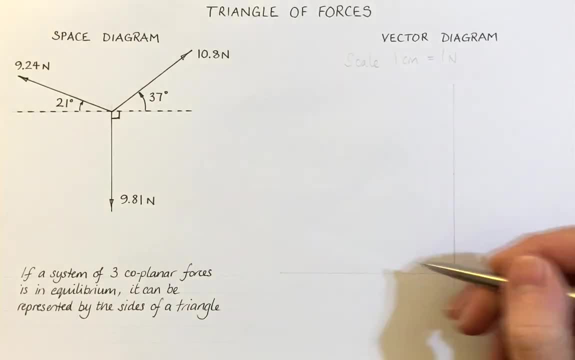 There's our first vector. It's acting straight down, So I'm going to show the direction. Now, if I put an arrow on the end, I run the risk of losing that accurate end point there. So I'm going to put the arrow, the direction arrow, halfway down. 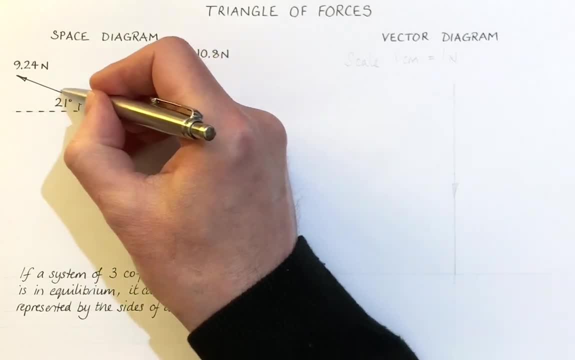 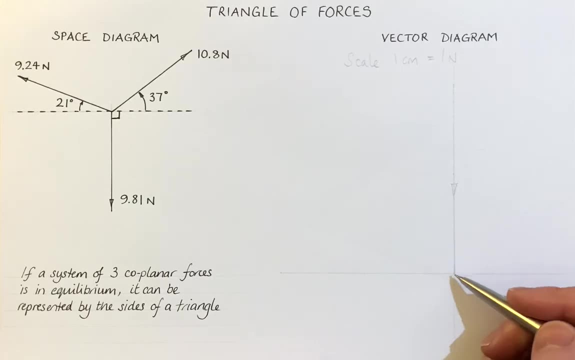 Next up, that's this one here. Next up, we're going to do this vector here. This is 9.24 newtons and it's acting up from the horizontal at 21 degrees, So it's going to go up in this direction here. 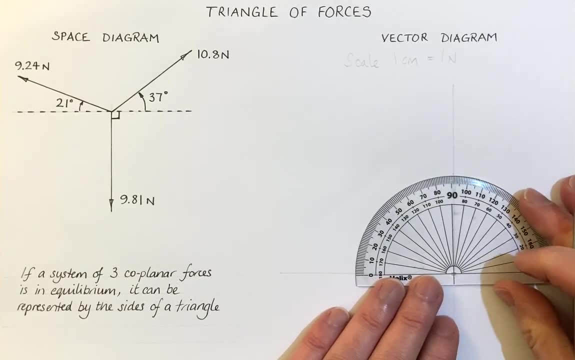 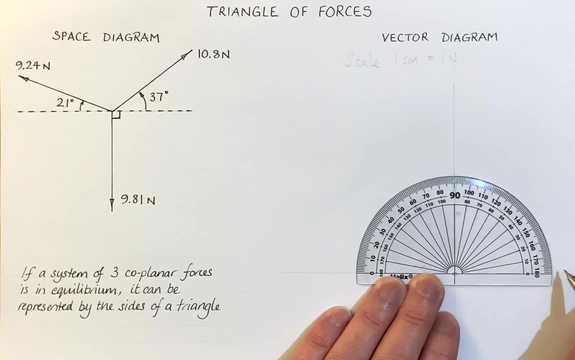 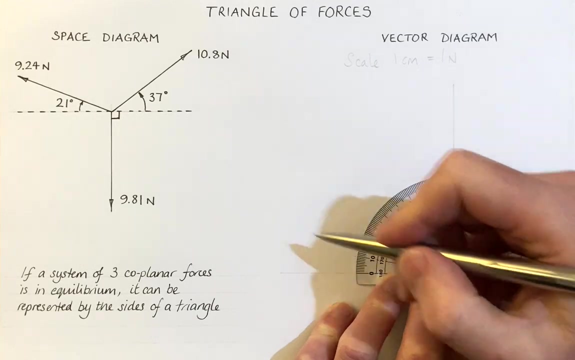 So I take my protractor Again and I put the crosshairs back on the origin there, carefully line up the zero here and zero on this side too. Oops, let's have another go. There we go, And I measure around 21 degrees. 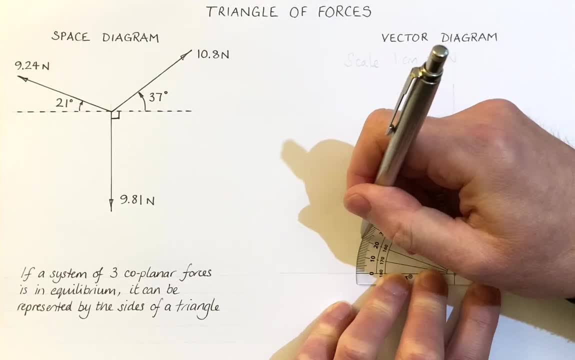 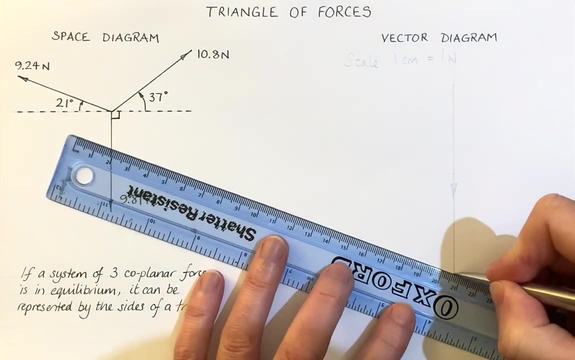 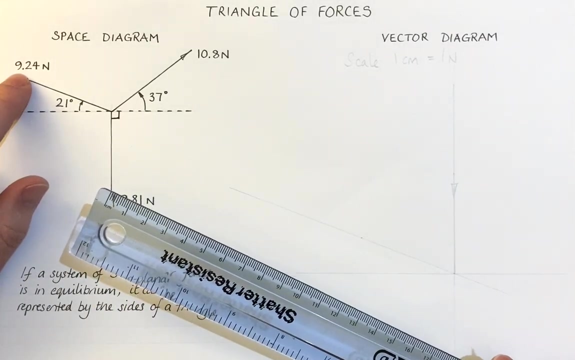 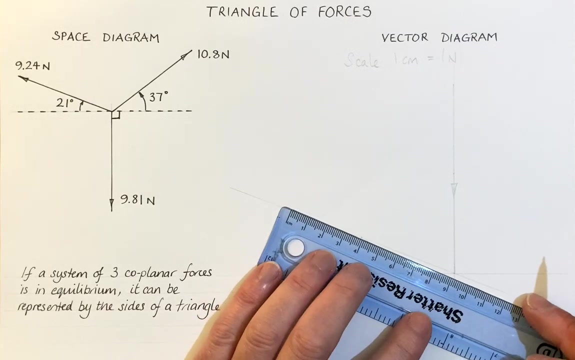 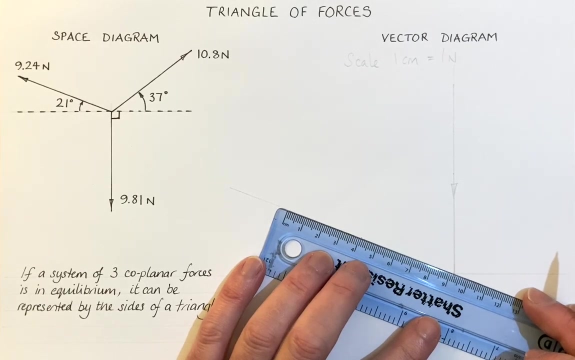 Here we go: 10,, 20,, 21 degrees. there Again, I'm going to draw a faint line first. There's our faint line first. Now, the magnitude of this vector is 9.24 newtons And because our scale is one centimetre to one newton, I'm going to measure 9.2,, something like 9.24, roughly halfway between those two marks there. 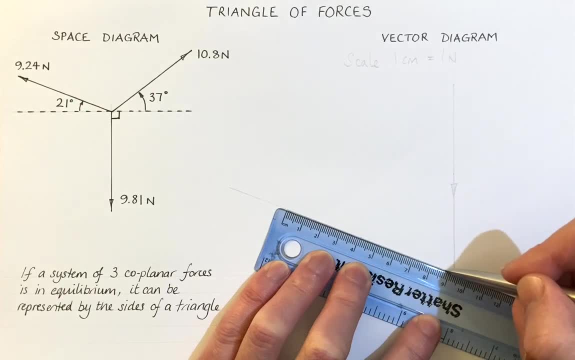 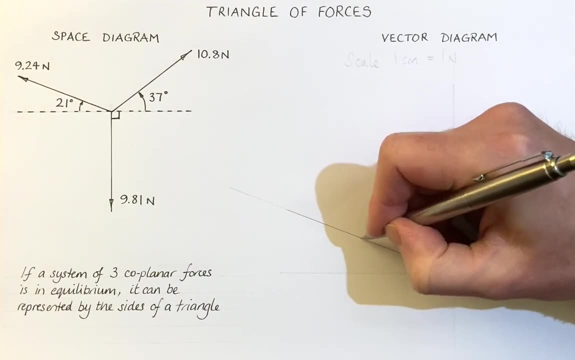 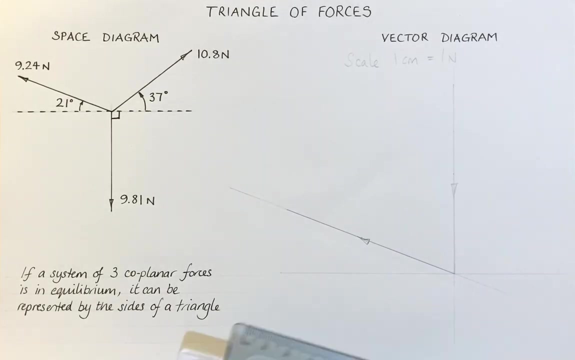 Here we go from the end. there There's our second vector and that's acting in that direction. So again, I'm going to show the direction here with an arrow. I've placed it in the middle. You can place it on the end if you like. 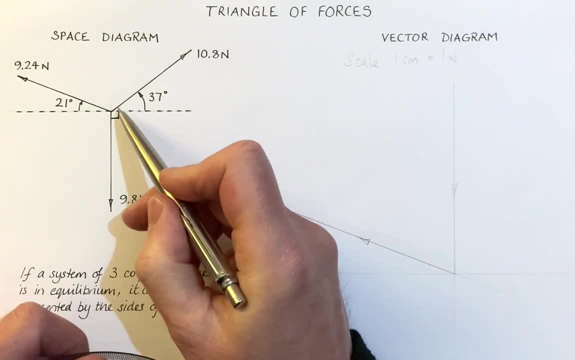 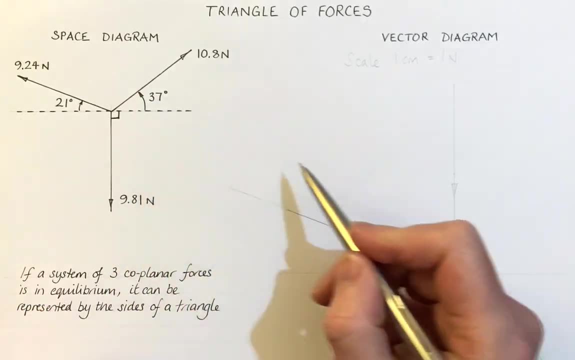 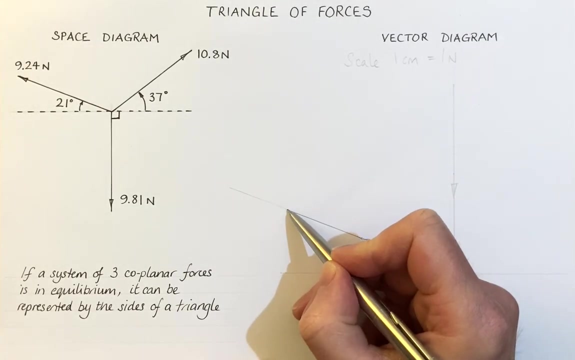 Now the next vector is this one here and that's 37 degrees up from the horizontal. Now I want to draw it from the end of this vector here back up to the top of the triangle There, But that angle there is not going to be 37 degrees. 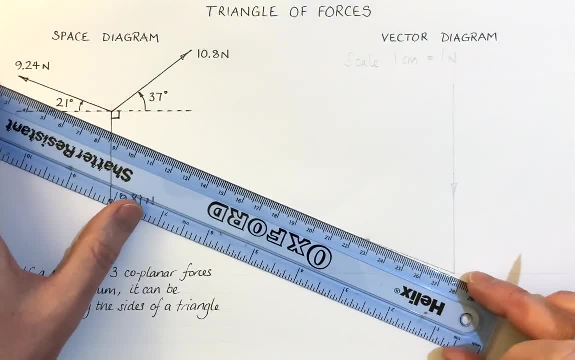 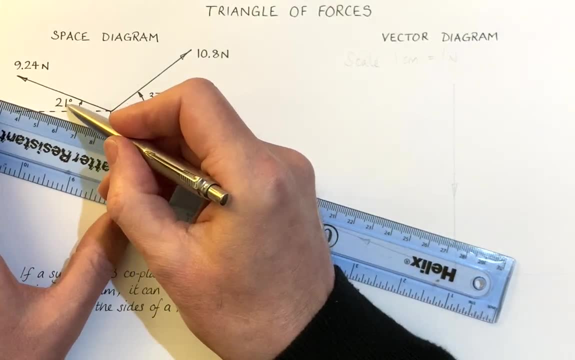 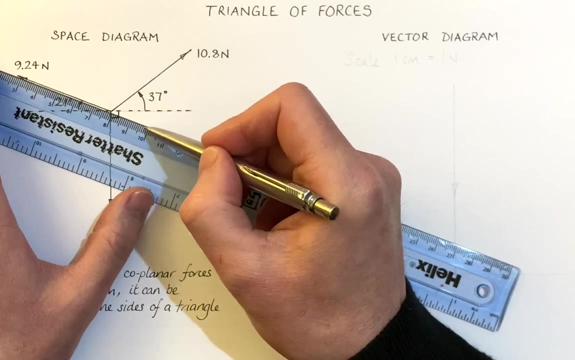 It's actually going to be a little bit more Now. if I place a rule on here, that angle down here is going to be the same as this angle here. So if that's 21 degrees, I know the total here is going to be 58 degrees. 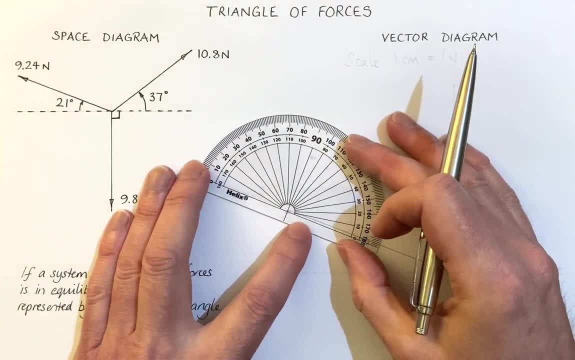 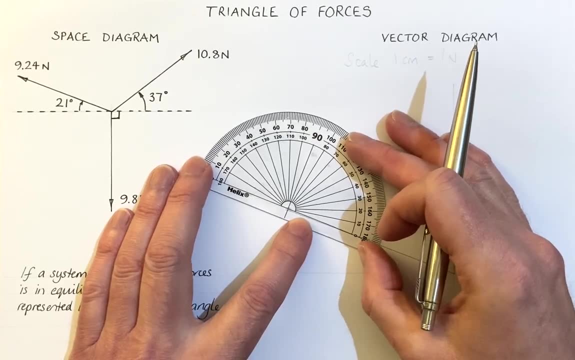 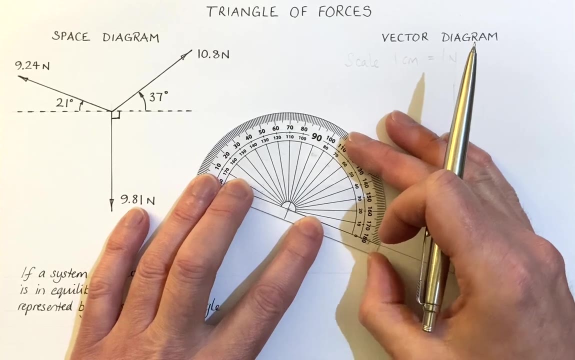 So I can put my protractor on The end of this line Here, making sure I get the crosshair on the end of the vector. There we go, Line up the zero there and that's going to be 58 degrees round from here.